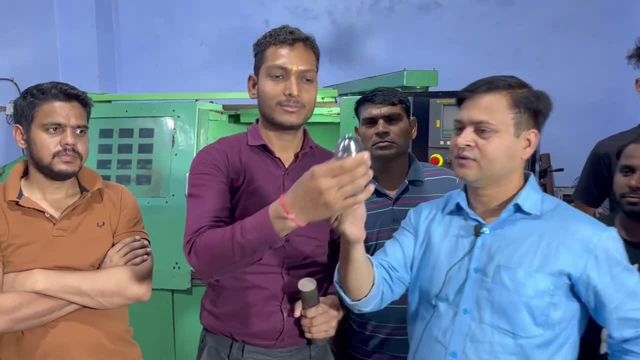 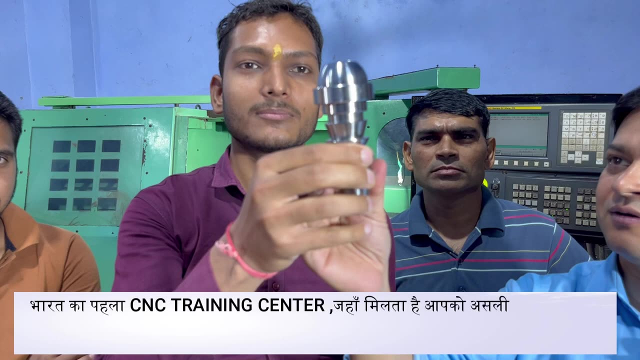 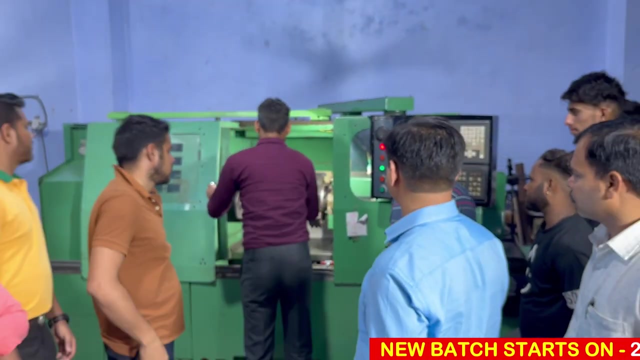 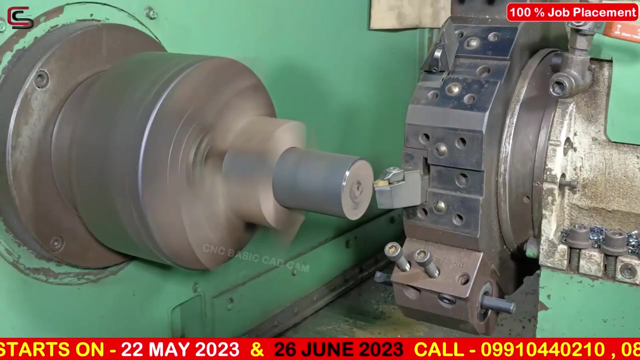 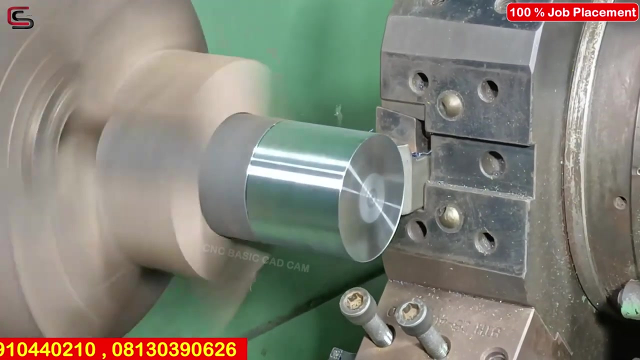 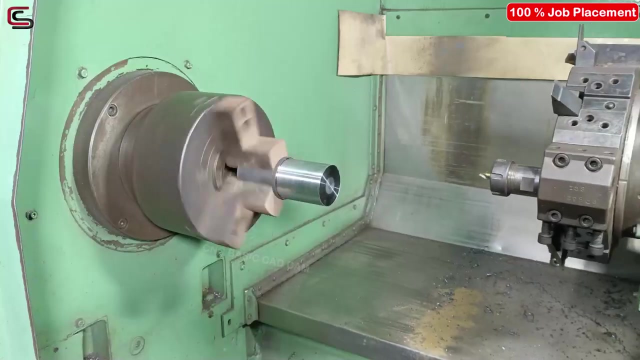 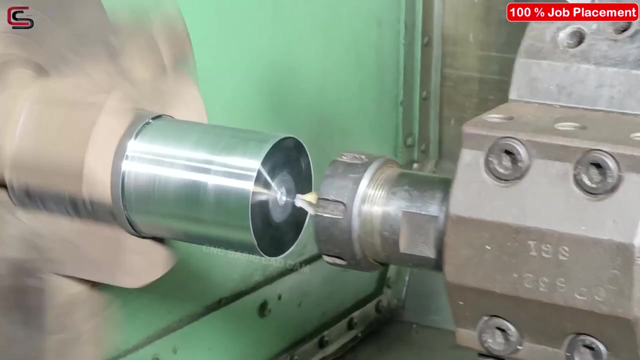 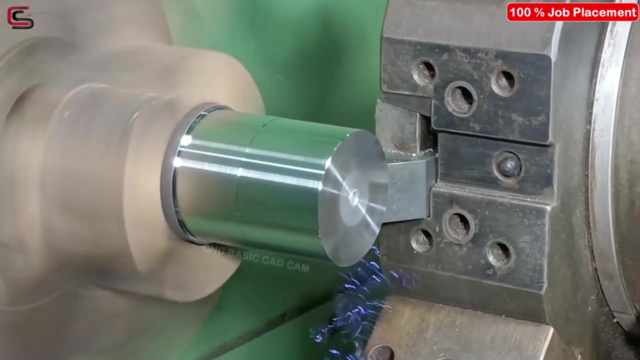 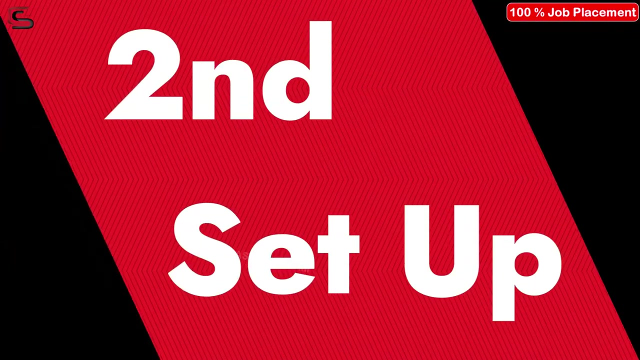 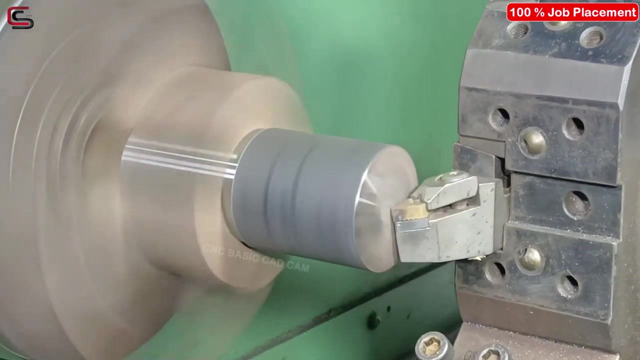 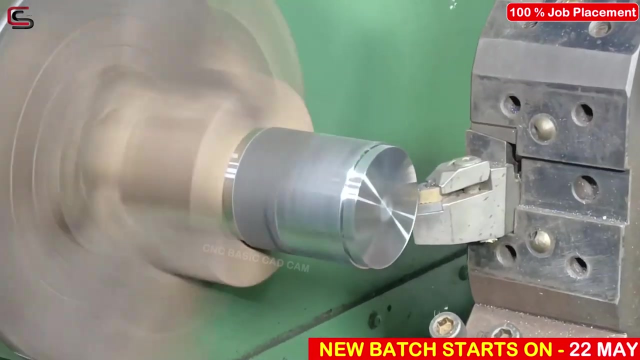 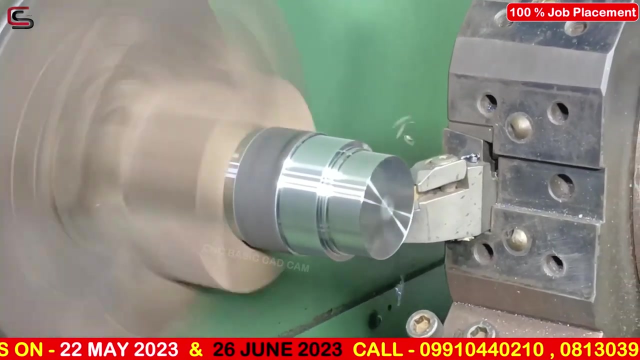 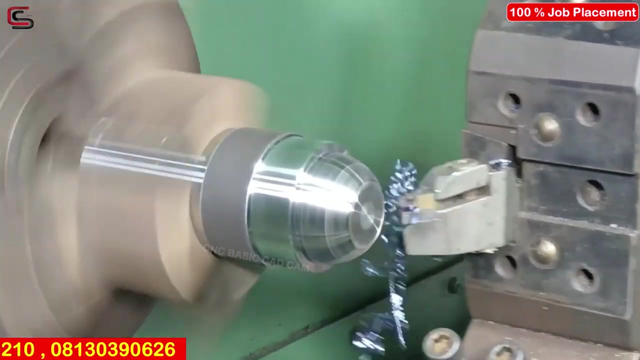 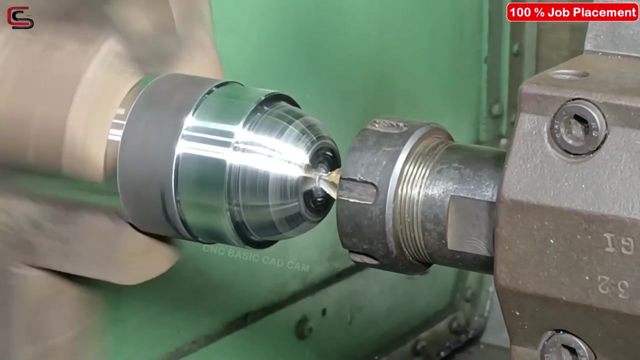 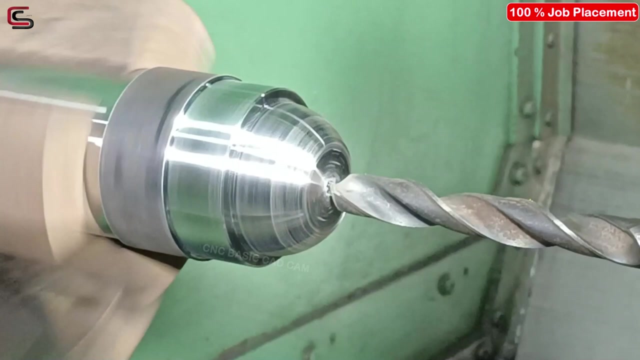 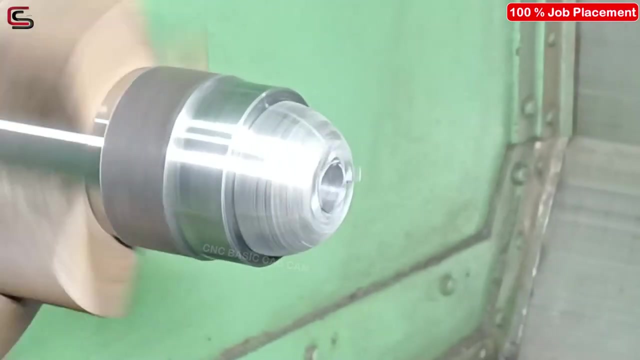 Come on, show us how this piece is made. Come on, show us how this piece is made. Hello everyone and welcome to cncbasicscom. I hope you are enjoying this video. In this video, I want to show you, guys, How to do the solution we need to do. 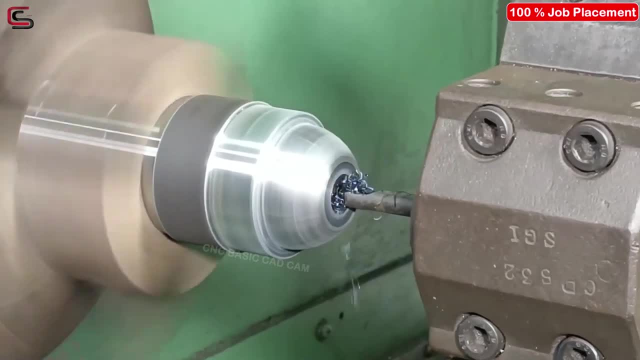 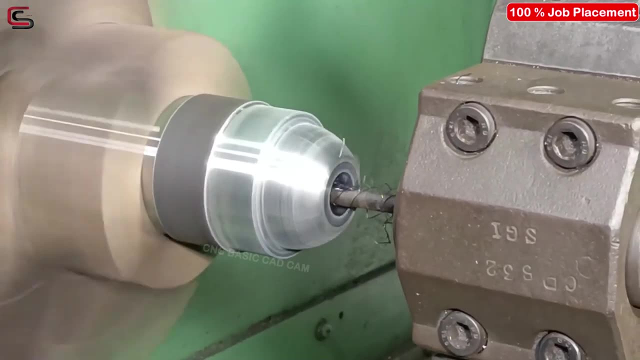 I have a dishcloth, I have a hat which is quite small, And I have a bag which is quite big, And I have a cup of tea, I have a cappuccino And I have a plate for our sauce, I have a can of shungiku.